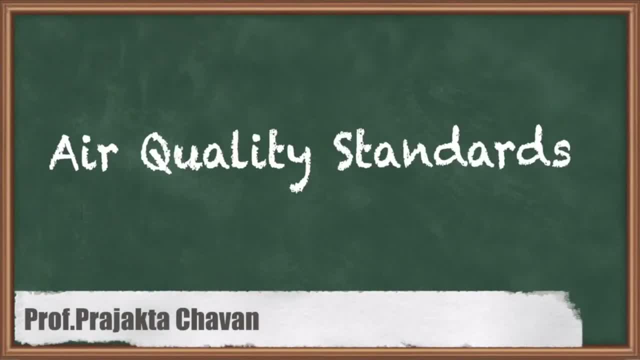 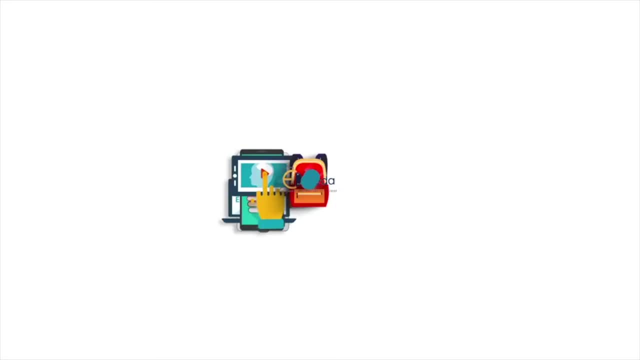 Hello everyone. In this lecture we are going to see air quality standards under the subject of environmental engineering. 1. So air quality standards that we are used to check the quality of air or purity of air And depending on that- that is quality of air- we are taking the action of control measures. 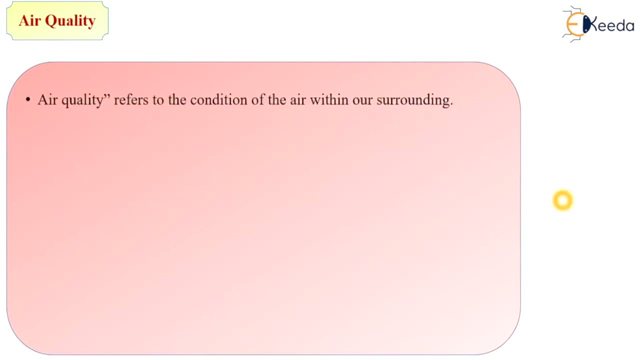 So what is air quality? Air quality refers to the condition of air within our surrounding. Good air quality pertains to the degree which the air is clean, clear and free from pollutants such as smoke, dust, smoke, among other gaseous impurities in the air. 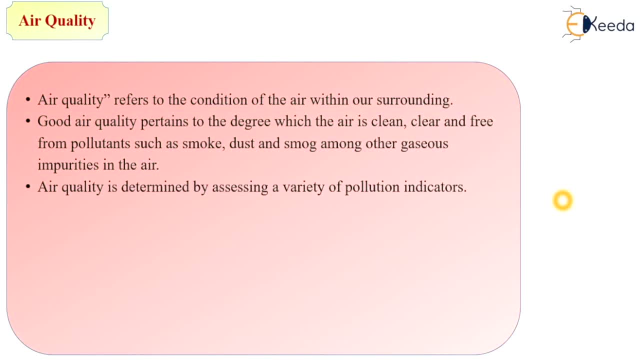 Air quality is determined by assessing a variety of pollution indications. Good air quality is requirement for: 1. Preserving the 2. Exigent balance of life on earth for human plant, animals and natural resources. At such human health, plants, animals and natural resources are threatened when pollution in the air reach the highest level or highest concentration level. 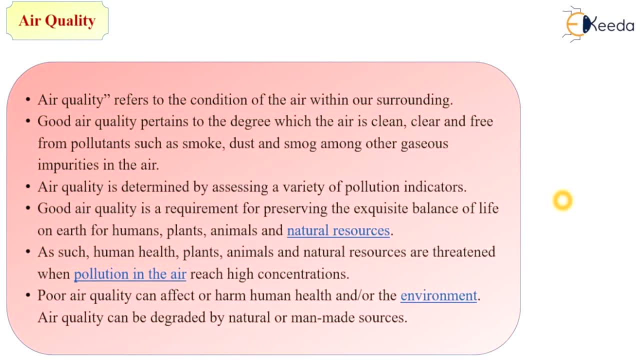 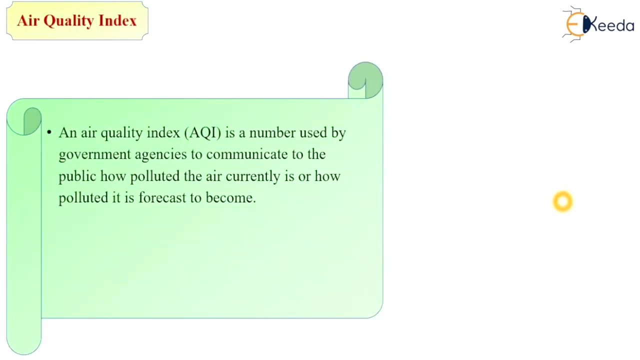 Poor air quality can affect or harm human health and or the environment. Air quality can be degraded by natural or man-made activities or sources. So for that, to check the quality of air, we are conducting or deciding the air quality standards. So next parameter that we are using to check the air quality is Air Quality Index. 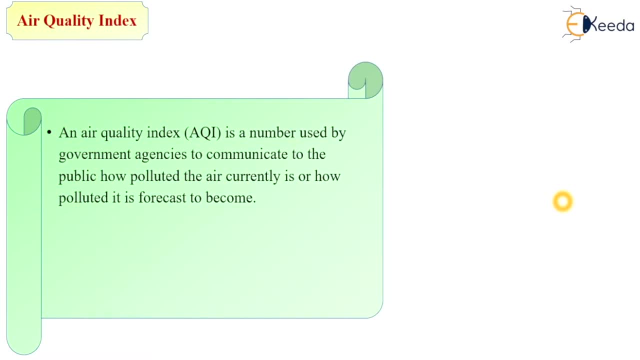 An air quality index is a number used by government agencies to communicate to the public how polluted air is. So air quality index is a number used by government agencies to communicate to the public how polluted air is- the air currently is, or how polluted it is forecast to be. so, as you all of know there, 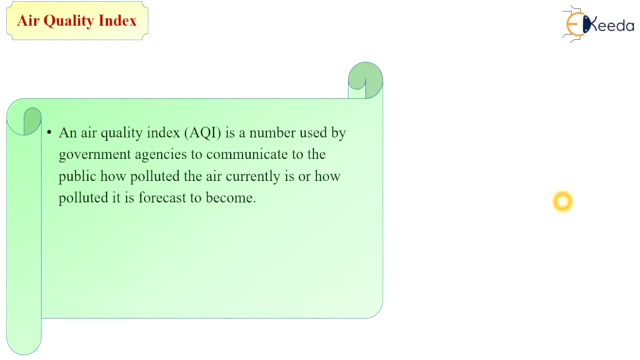 are some water quality standards or wastewater quality standards. so we are representing that quality of water or wastewater in terms of some values. so, similarly, in this way, for checking the air quality, there is a air quality index which represent a number and on basis of that number we are deciding that or we are considering that, that the air, present condition of air, is. 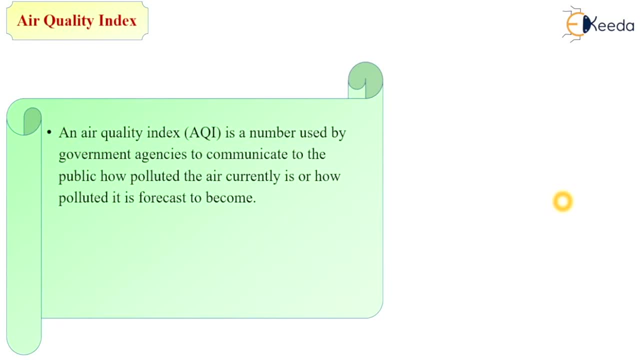 how much polluted, or whether it is clear or whether it is polluted. so as the air quality index increases, an increasingly large percentage of the population is likely to experience increasingly severe adverse health effect. that means that when the number is increasing, the pollution is increasing or it represents. 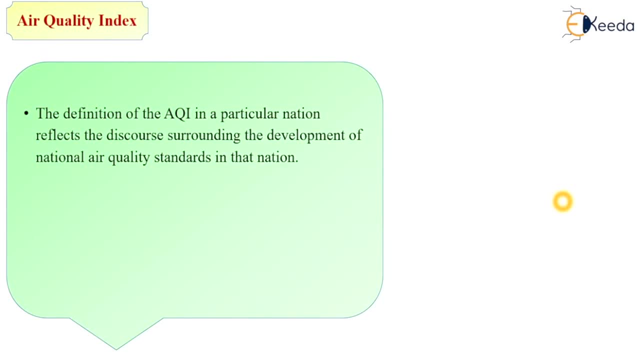 the polluted air. So the definition of air quality index in a particular nation reflects the discourse surrounding the development of national air quality standards in that nation. Most air contaminants do not have an associated air quality index. Many countries monitor ground level ozone, particulate matter, sulfur dioxide, carbon monoxide and nitrogen. 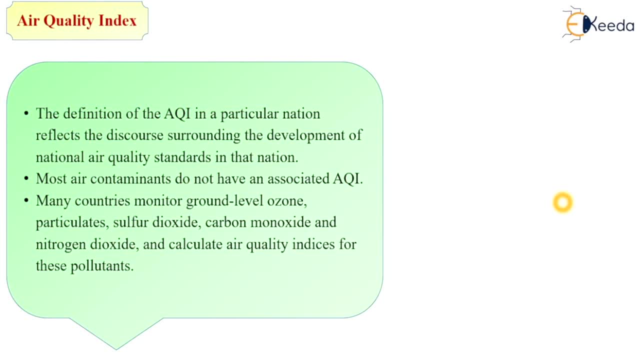 dioxide and calculate air quality indices for the pollutants. So these are the main contaminants or impurities that are present in air, which are present in nature and which are toxic in nature when it increases its permissible limit, because these primary or secondary pollutants present in air are very minute level or very minute quantity. So if 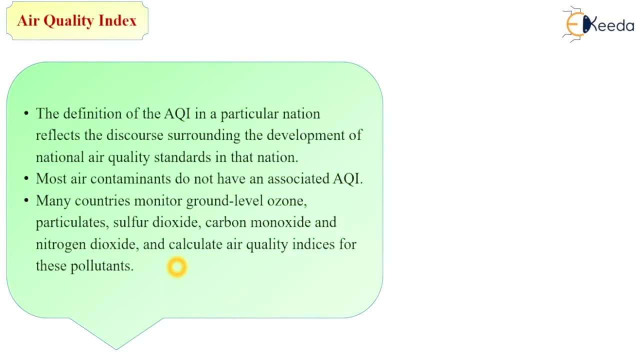 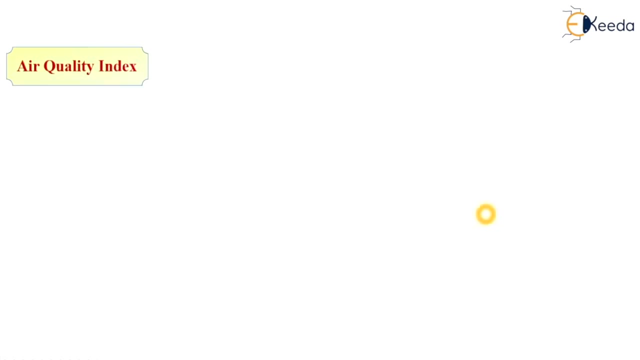 their limit is exceeded, then it will adversely impact the air quality index. So this is the effect on human health, as well as on properties or buildings, So that by considering these primary or secondary pollutants, the air quality indices is decided for to check the quality of air. So on a day when air quality index is predicted to be elevated due to the 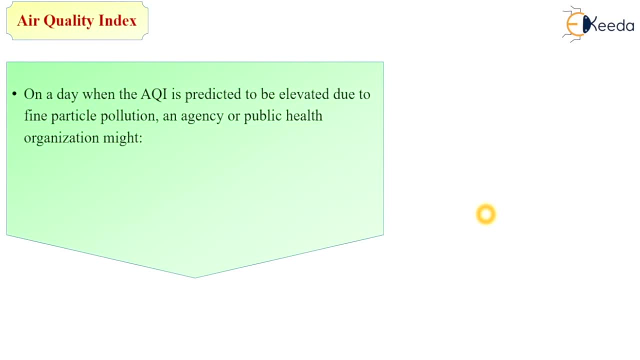 fine particle pollution. an agency or public health organization might advise sensitive group such as the elderly, children and those who are in the public health organization with respiratory or cardiovascular problems to avoid outdoor exertion. Again, declare an action day to encourage voluntary measures to reduce the air emissions, such as using 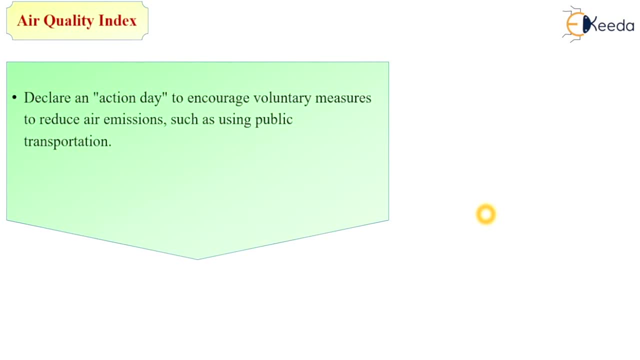 public transportation. So, as we learnt in previous lectures, that is air pollution or air pollutants. So carbon monoxide is very toxic pollutant that is emitted from the vehicular transportation. So we have to control on the emission of this carbon monoxide, That is. 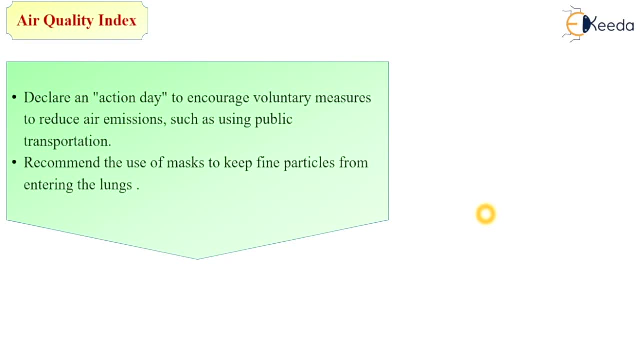 why we recommend the use of mask to keep fine particles from entering the lungs. So every time we cannot control to reduce this emitting of air pollutants from the source. So the other way of controlling this effects is to providing or to keep the mask on your face. 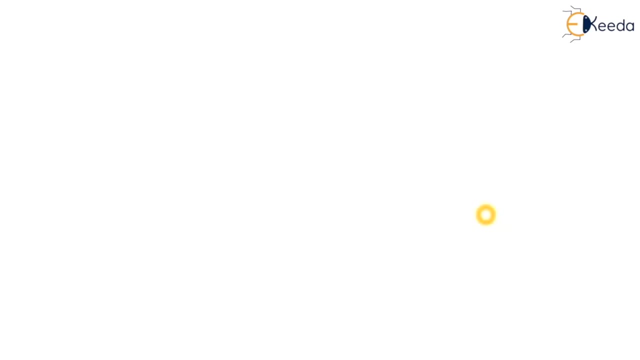 to avoid the entry of fine particulate matter into your nose or lungs. The silent features of the air quality index are: The measurement of air quality index is based on 8 pollutants that are particulate matter 10, particulate matter 2.5. So that 10 and 2.5 are the size of that particles in micrometer. 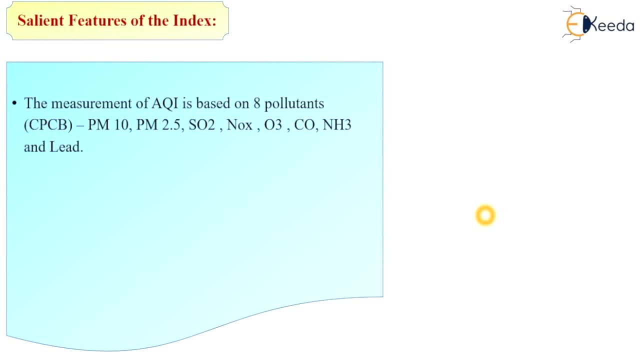 Then SOX, NOX, that is SO2,, NOX, that is oxides of nitrogen, O3, that is ozone, CO, that is carbon monoxide, NH3, that is ammonia and lead. So these are 8 pollutants and these are based. 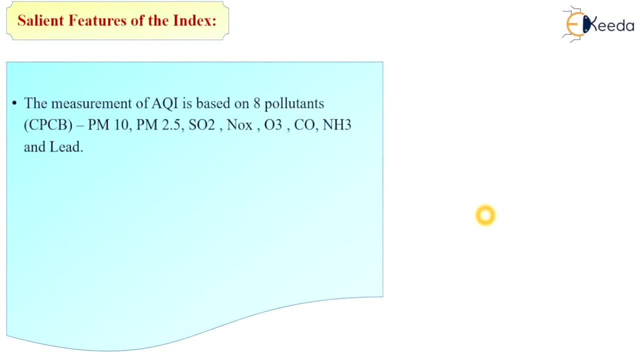 on the air quality index And depending on or that basis we are taking the measurements of air quality index. The unit of measurement is microgram or milligram in the case of carbon monoxide per cubic meter. So many times you have asked questions in objective, like what: 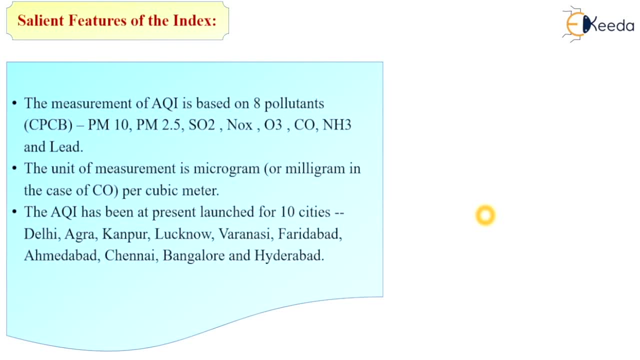 is the unit of measuring the air pollutants, that is in micrograms. The air quality index has been at present launched for 10 cities, that is, Delhi, Agra, Kanpur, Lucknow, Delhi, Varanasi, Faridabad, Ahmedabad, Chennai, Bangalore and Hyderabad. So these are the 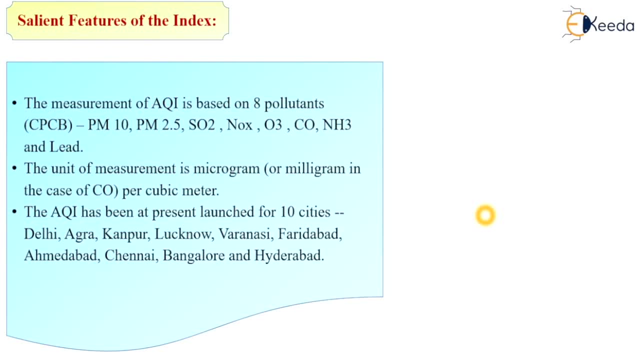 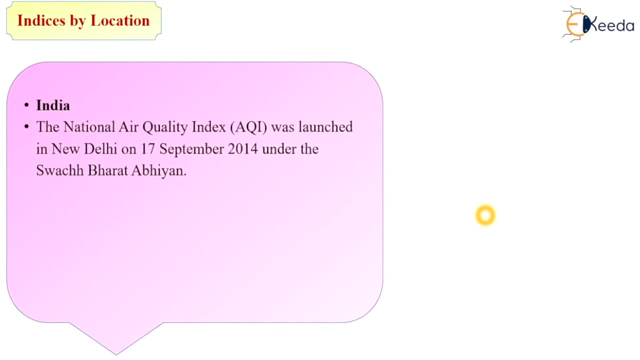 most polluted regions. air polluted regions, So that we are considering that 10 cities. So indices by location. So we will see the indices. air quality of India. The national air quality index was launched in New Delhi on 17th September 2014.. Under the 17th September: 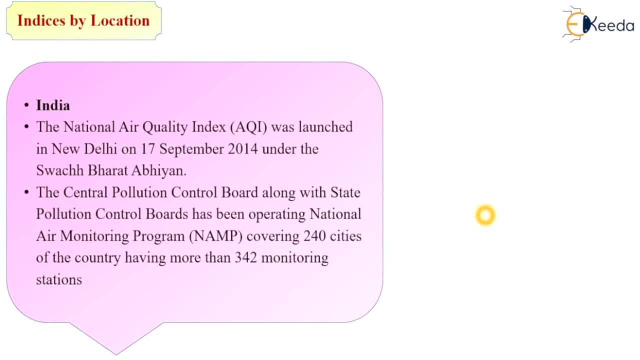 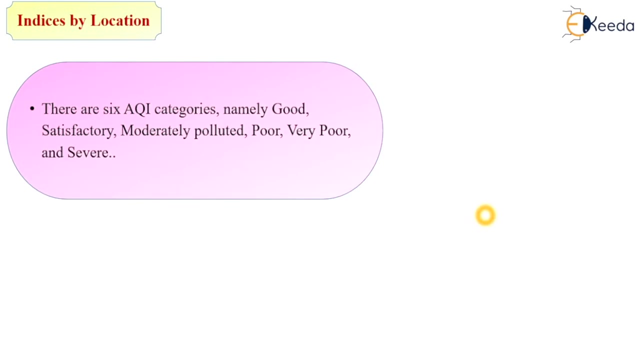 2014,. the central pollution control board, along with state pollution control board, has been operating national air monitoring program covering 240 cities of the country having more than 352 monitoring stations. So there are 6 air quality index categories, namely good, satisfactory, moderately polluted, poor, very poor and severe. So, depending on the 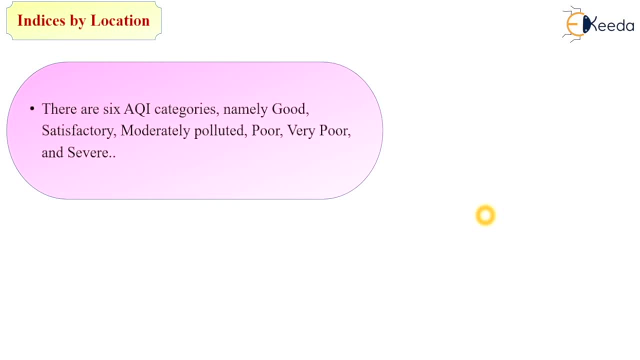 representation of the air quality index. we are considering that 10 cities of the country are highly polluted and very severe. So under the number 9,, 7 or higher, we are deciding that whether the air quality index is good in nature, satisfactory in nature, moderately. 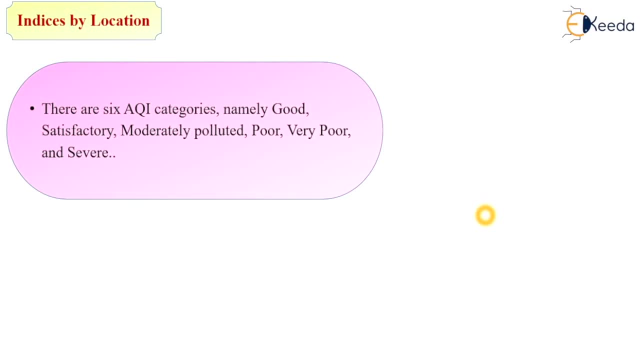 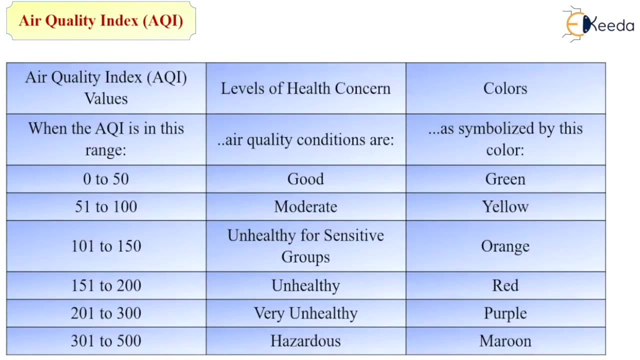 polluted, poor, very poor and severe. So let's we see the actual values of air quality index. So, as you can see in this table, the first column representing the air quality index values, second column representing the levels of health concern, ie which will 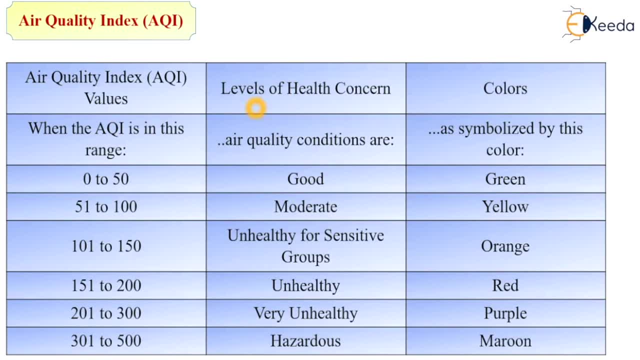 you affect, at what percentage of health effect? and last one is the color, the indication of color of that air present in atmosphere. For example, when the air quality index is in this range, that is, 0 to 50,, then the air quality conditions are good. So, as you can, 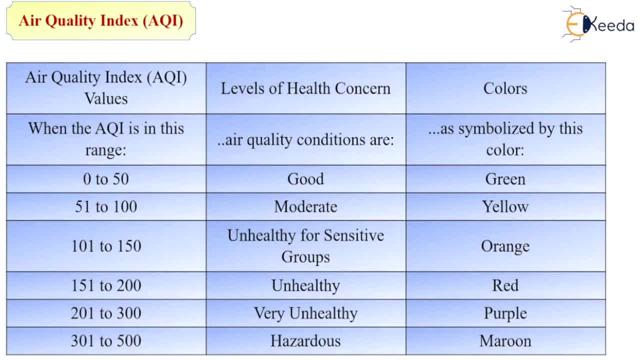 see the values are starting from 0 and end up to 500. That means the range is category, as first is 0 to 50, then 51 to 100, then 101 to 150, 151 to 200, 201 to 300 and 301. 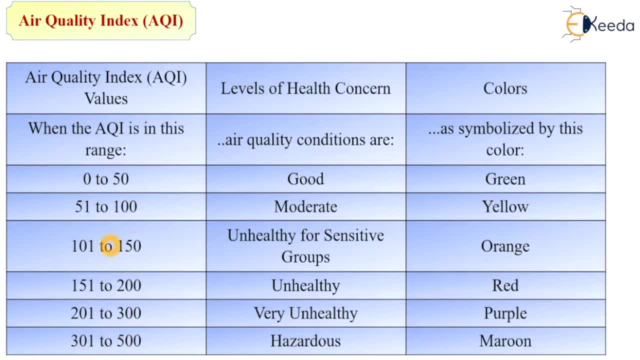 to 500.. So by the difference of 50, we are categorize these values. So first is 0 to 50. If air quality index value is present in between 0 to 50, then the range is 0 to. 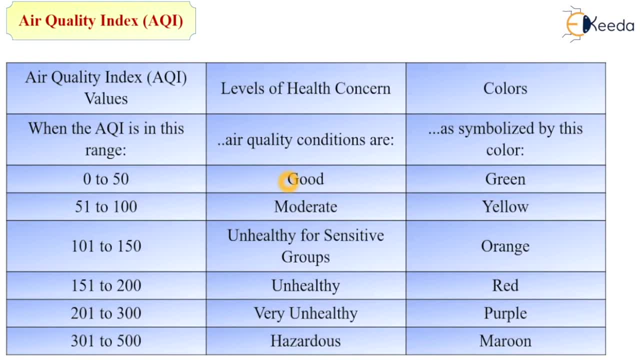 50. If air quality index value is present in between 0 to 50,, then the quality, the conditions of air present in atmosphere is good and the color of, as symbolized by this color, the color of air or atmosphere, is represented as green. That is the reflection of nature. 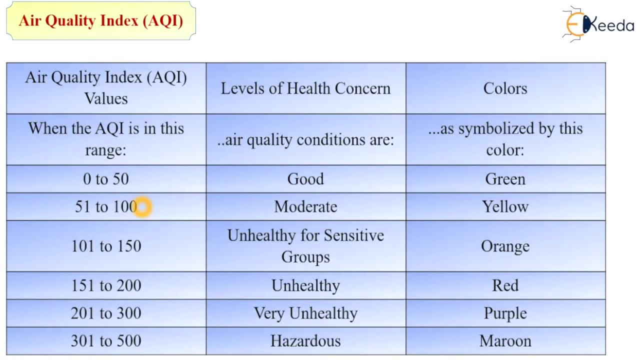 or reflection of plants. If this value is little bit exceeded, that is 51 to 100, then the quality of air is moderate and representation of color of atmosphere is yellowish in nature. If further this value is exceeded, from 101 to 150, so that condition might be unhealthy. 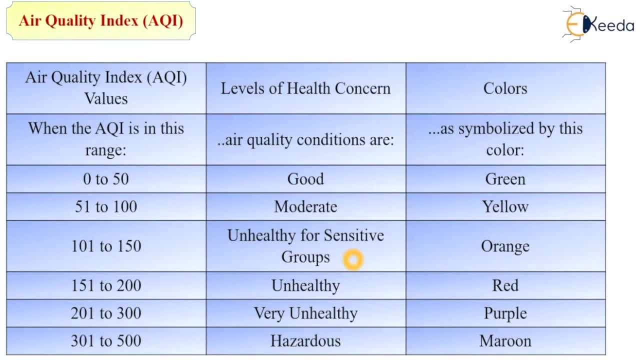 for sensitive groups. So sensitive groups means the aged group of people or children, and in that conditions the color is color, reflection is represented of atmosphere, is orange in nature. So next, again, this value is in the range between 151 to 200, then the 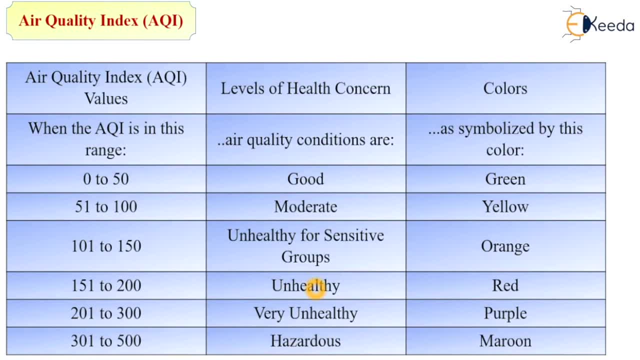 quality or condition of air is unhealthy type And the representation of color is red. Again, this value is exceeded up to 300, then the condition become very unhealthy and the atmospheric reflection, color reflection- is purple in nature And the last one, that is very severe condition. that is the value is presenting. 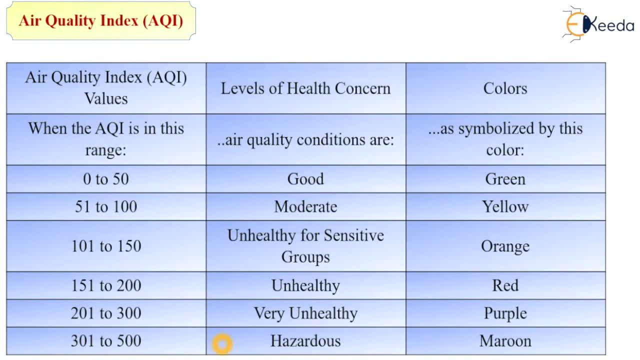 between 301 to 500. So in that state this is the last stage of polluted air. that means the condition of air is very hazardous. So, and the color is red. So if this value is higher, we can see that then it is not considered the color of the air In the case of this. 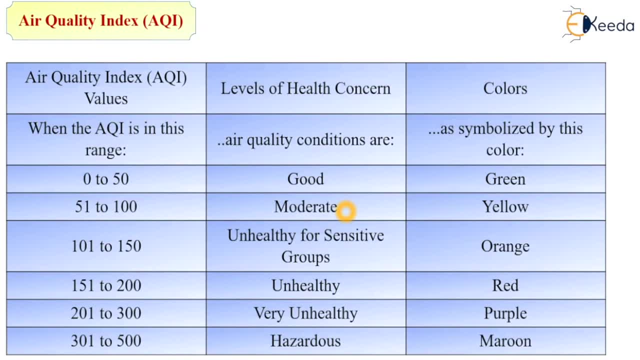 example, we have this colour reflection represented as maroon in color. So up to moderate condition, we will what you say. we will accept the condition of air, or we are susceptible or suspecting to this, or environment or the atmosphere. But once this condition is increasing and 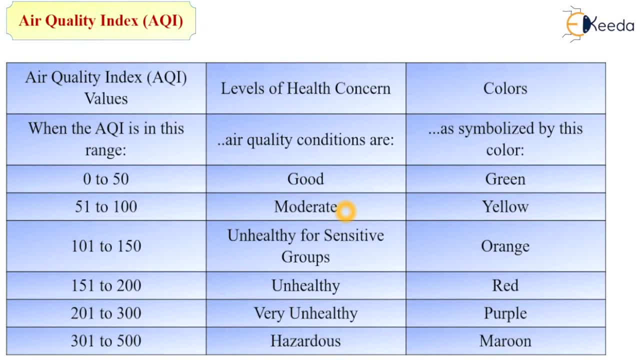 reach up to the very unhealthy and hazardous conditions, then we have to, or we must have to, put some control measures on that condition that we are not sensitive to this environment and we are not able to take this, as that is one of the most permanent hard factors. 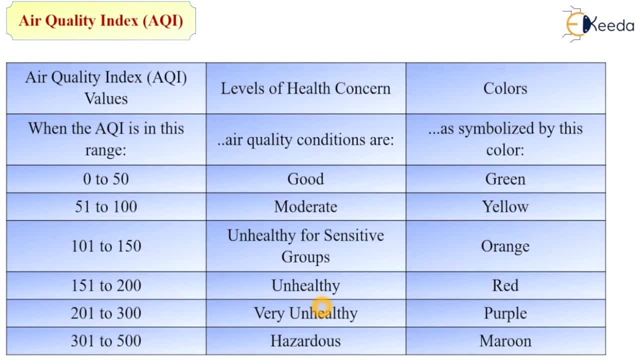 So last one, that is, the next condition, is that we are not able to go in the air So immediately. we are in a very difficult situation Because we are not able to move, otherwise reduce the quality of air or to reduce- sorry, to reduce- the pollution of air or to reduce. 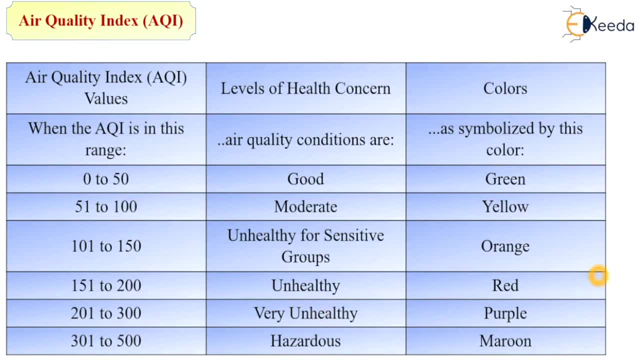 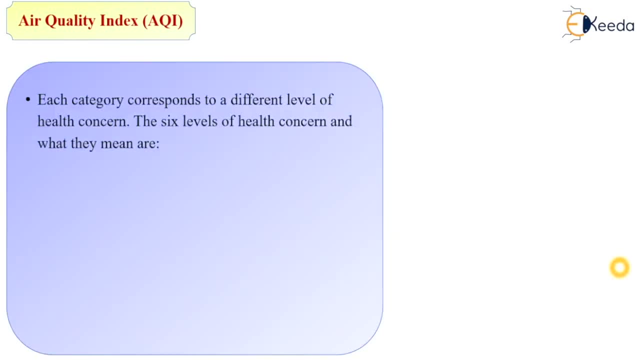 the concentration values of air pollutants and because of that the air will get polluted. so next, each category corresponds to a different level of health concern. the six level of health concern and what they mean are: the good condition of air quality index is value up to 0 to 15. 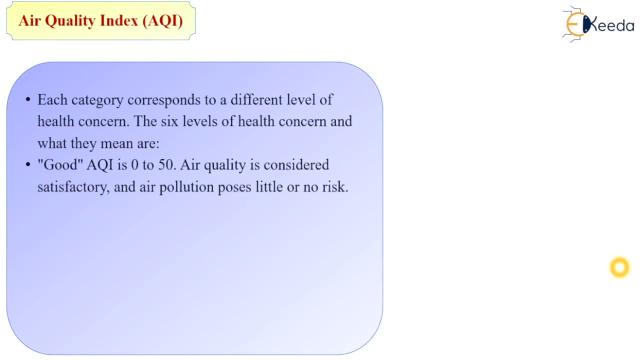 so the air quality is considered satisfactory and air pollution pose like or no risk. in moderate condition the air quality index value is 51 to 100. that means the air quality is acceptable. however, for some pollutants there may be a moderate health concerns for a very small number of people. for example, people who are unusually sensitive to ozone may experience. 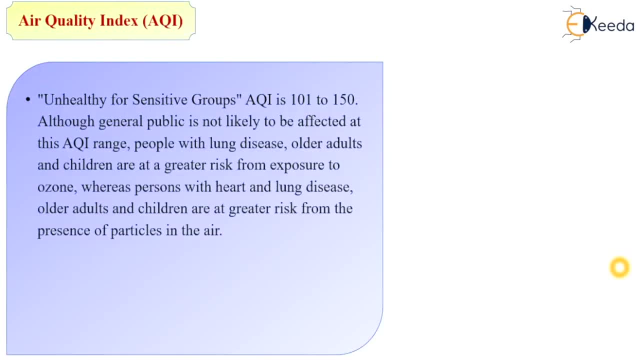 respiratory symptoms. next number is next condition is unusual for sensitive group. for that the air quality index value is 101 to 150, although the general public is not likely to be affected at this air quality index range, but the people with lungs disease- older adult group, the childrens- are at a greater risk from exposure to ozone. 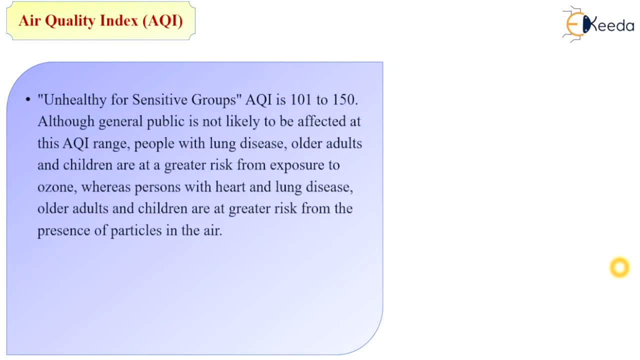 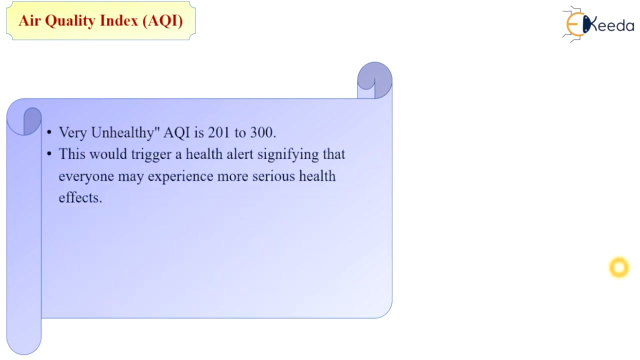 whereas person with the heart and lungs diseases, older adult and childrens are greater risk from the presence of particles in the air. so next is unhealthy condition for that the air quality index is 151 to 200, so everyone may begin to experience some adverse health effect and number of the sensitive group may experience more serious effect when the air quality index values is reached up to the unhealthy condition. and second last is very unhealthy condition for that the air quality index value is 201 to 300, so this would pre-convert to the unhealthy condition. and the second last is very unhealthy condition for that: the air quality index values 201 to 300, so this would pre-convert to the unhealthy condition. and the second last is very unhealthy condition for that the air quality index values 201 to 300, so this would pre-convert to the unhealthy condition. and the second last is very unhealthy condition for that the air quality index values 201 to 300, so this would pre-convert to the unhealthy condition. and the second last is very unhealthy condition for that: the air quality index values 201 to 300, so this would pre-convert to the unhealthy condition. and the second last is very unhealthy condition for that the air quality index values 201 to 300, so this would pre-. 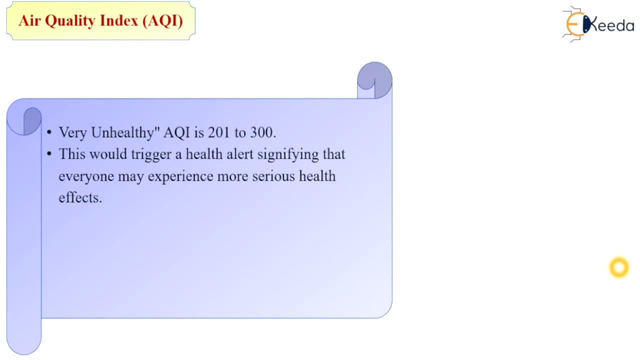 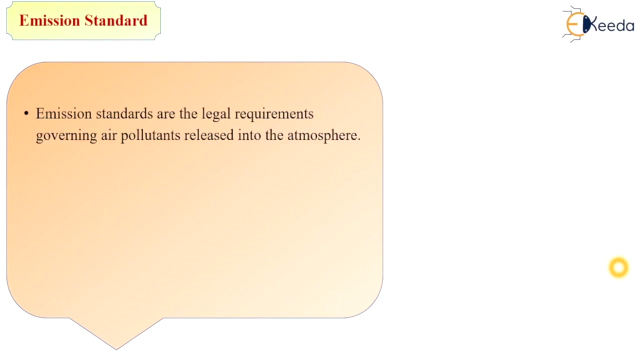 healthy condition for that. the air quality index values 201 to 300. so this would pre- healthy condition for that. the air quality index values 201 to 300. so this would pre- healthy condition for that. the air quality index values 201 to 300. so this would pre-. 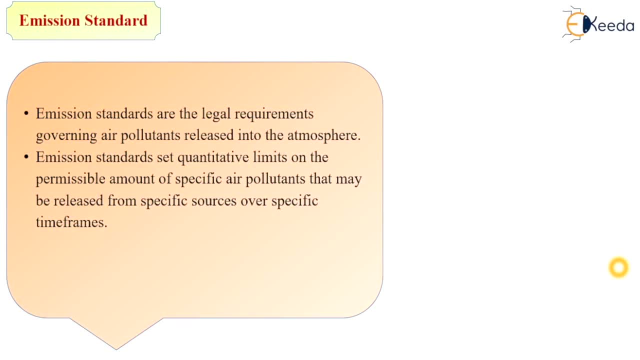 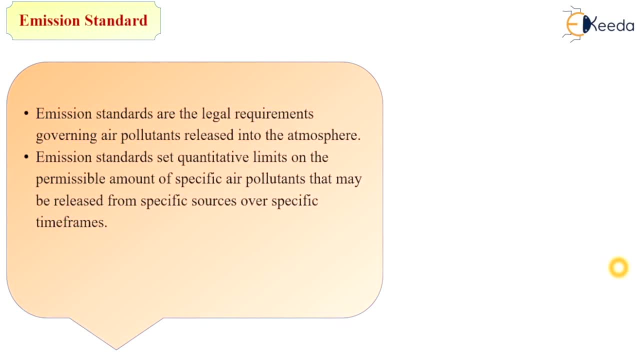 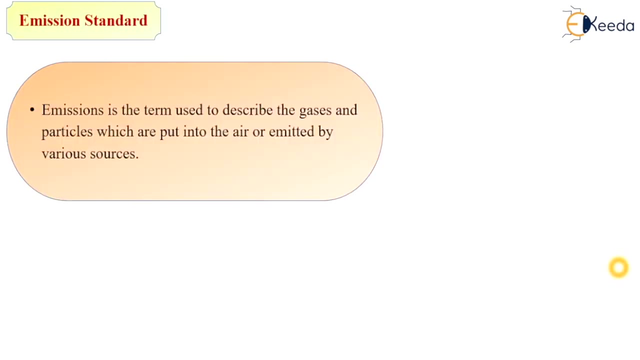 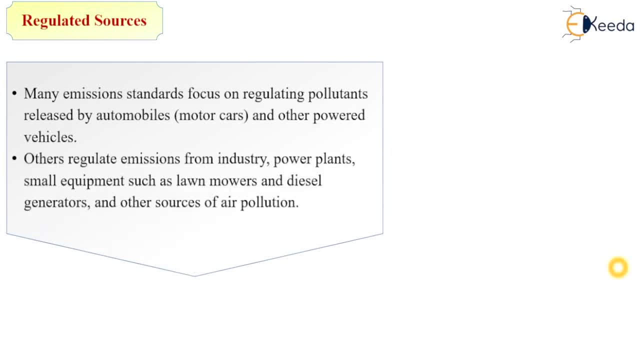 of automobiles, ie motor cars and other power vehicles. The others regulated emissions from the industry, power plants, small equipment such as lawn mowers and diesel generators and other sources of the air pollution. So these are some sources of emission of air pollutants. 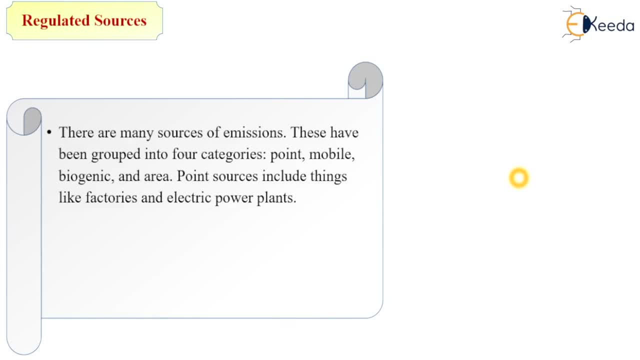 There are many sources of emissions. These have been grouped into four categories: The prime source, mobile source, biogenic source and area source. Pond source includes things like factories and electric power plant, So in pond source the pollutants are directly emitted from this source. 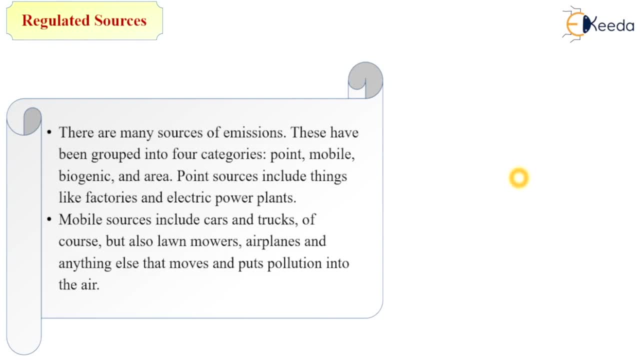 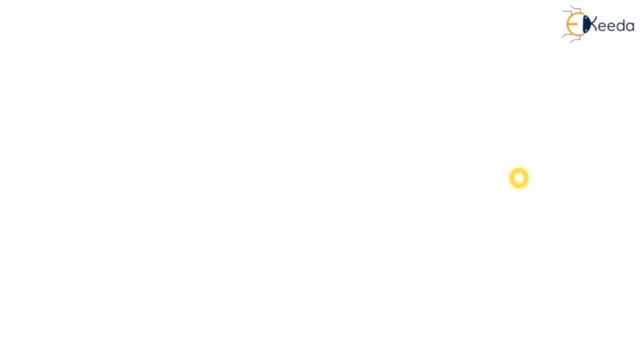 Mobile source includes the cars and trucks, So that means the pollutants are released when these sources are movable in nature, Of course, but also lawn mowers, aeroplanes and anything else that moves and puts pollution into the air, So these are considered the movable sources.